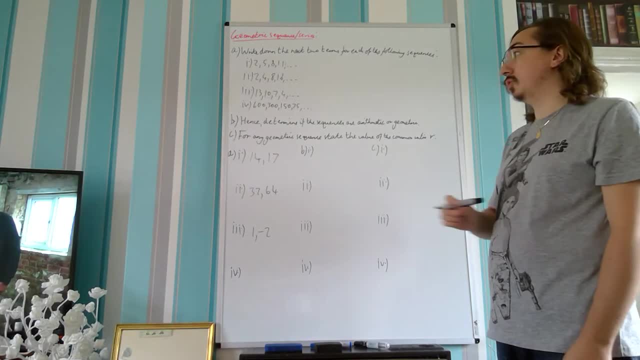 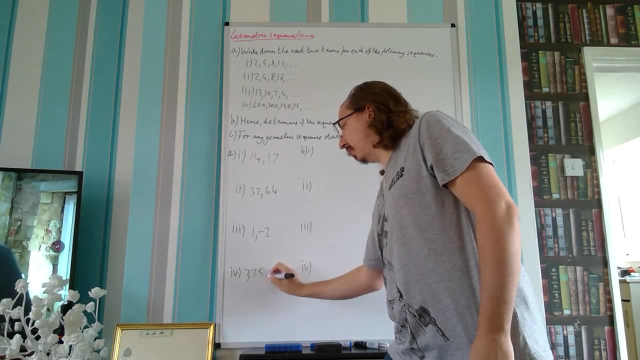 same as multiplying by a half, and that will become important shortly. But if we're dividing by 2, each time, 75 divided by 2 gets us 37.5.. 37.5 divided by 2, 18.75.. Obviously, you'd. 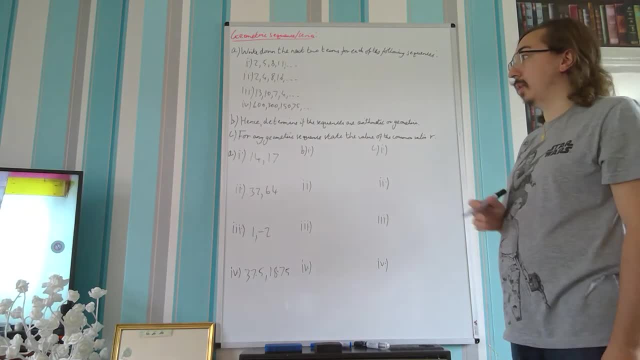 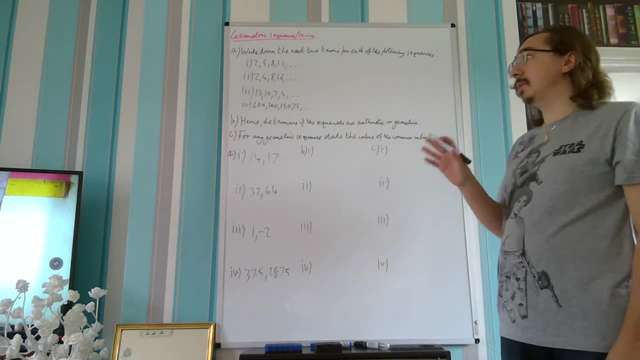 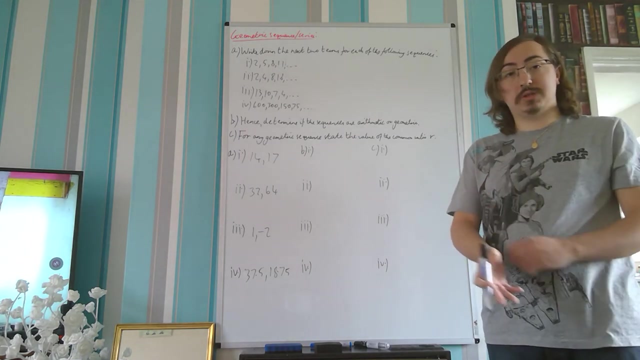 be fine to write those as fractions, but decimals are quite nice when you're writing them in. Decimals are quite nice for this particular problem. So we've got our next two terms, for each of the sequences Part says to determine, hence determine if the sequences are arithmetic or geometric. So that comes back to our definition. 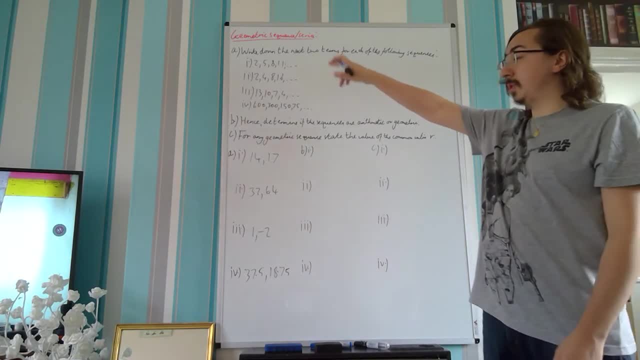 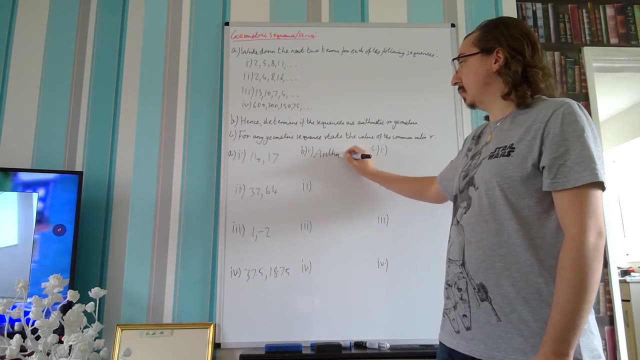 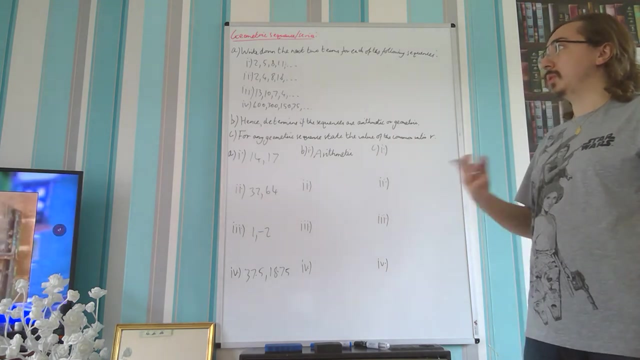 of the type of sequences. So for our first sequence, because we are adding each time, that makes this an arithmetic sequence, So it's an arithmetic sequence. For the second sequence, we're going: 2 times 2 is 4 times 2 is 8 times 2 is 16, and so on. 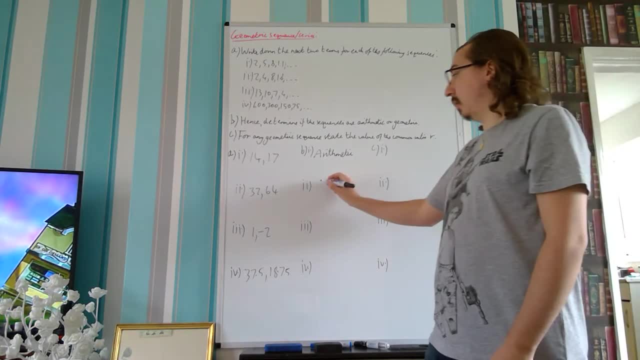 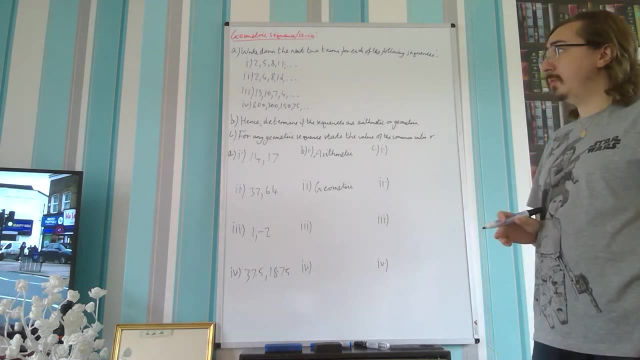 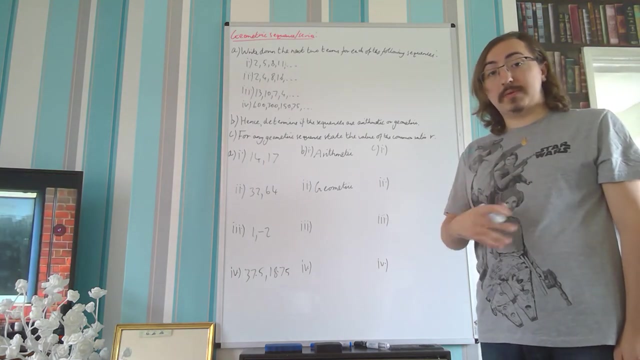 So, because we are multiplying each time, this makes it a geometric sequence. For the third one, which is 13,, 10,, 7,, 4, and so on, each time we are subtracting 3.. And if it's a subtraction, 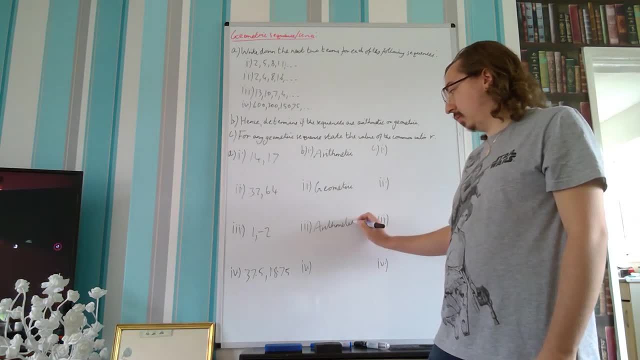 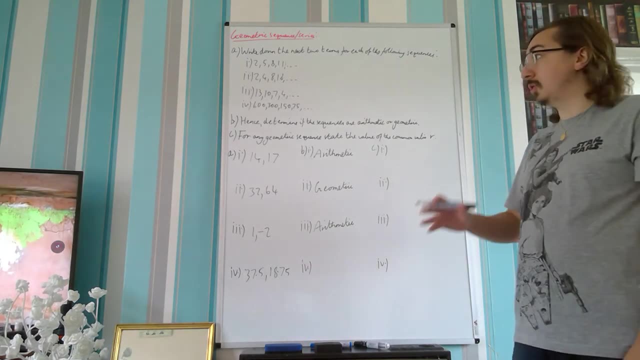 this makes it an arithmetic sequence sequence. And for the last one, 600, 300, 150, 75. So we're dividing by two each time, or, as I said, importantly times in, by a half. So because there is a multiplication, 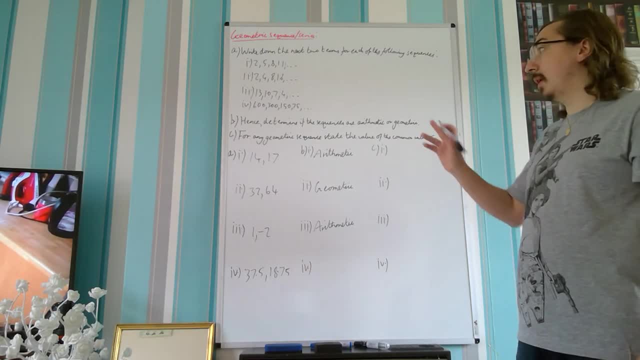 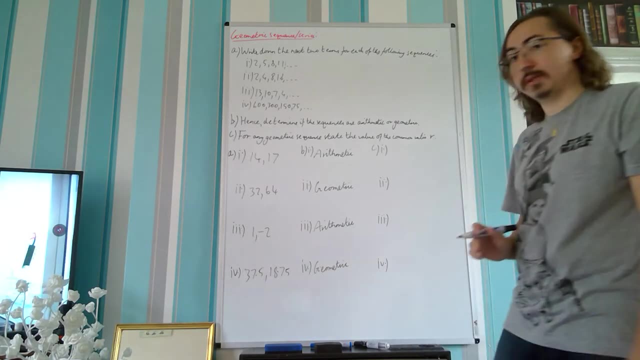 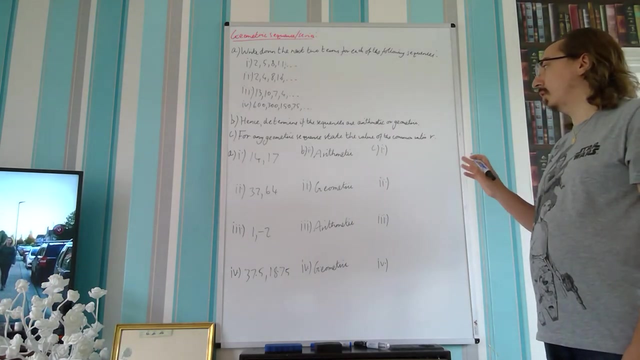 there or a division, depending on which way you want to view it. that makes this a geometric, Geometric. So this is a geometric sequence. So part C says for any geometric sequence state, the value of the common ratio R. Well, the first one is an arithmetic, so we can. 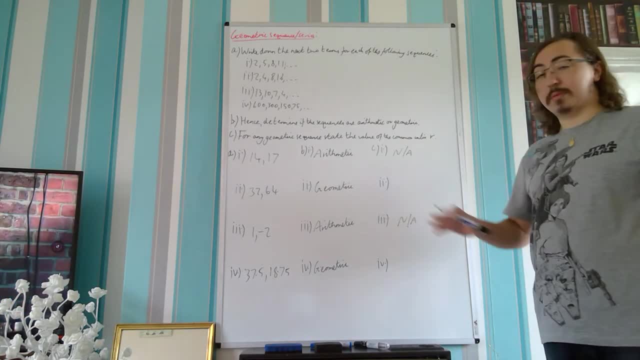 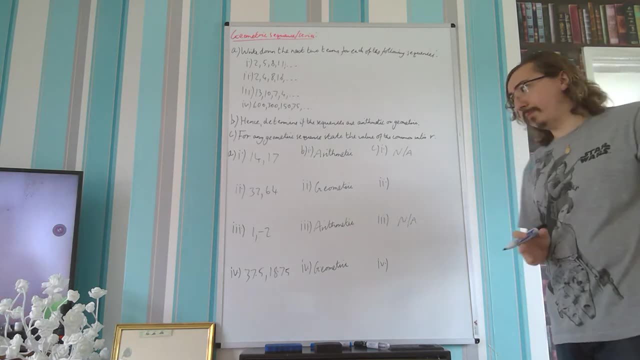 say that's not applicable. and the same for the third one, because they're both arithmetic and we've already discussed. for this one we're adding three each time. This one we're subtracting three each time. For our geometric we're adding three each time, So we're adding.